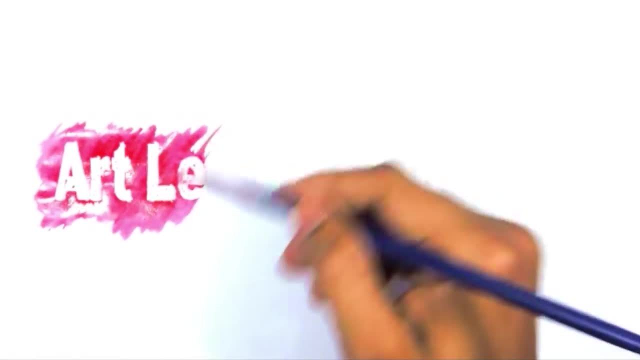 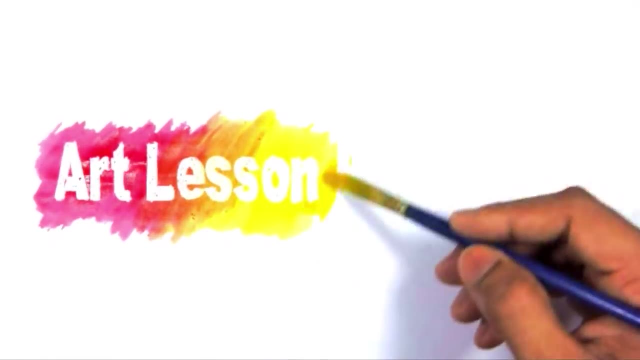 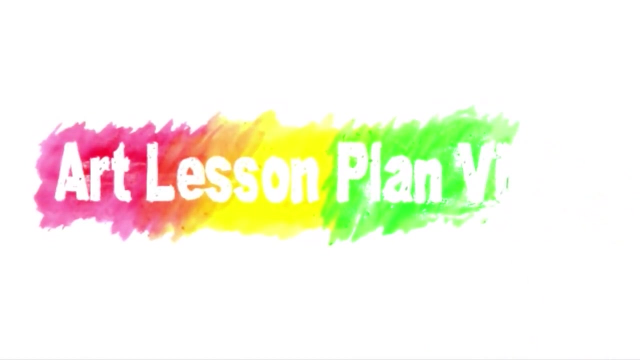 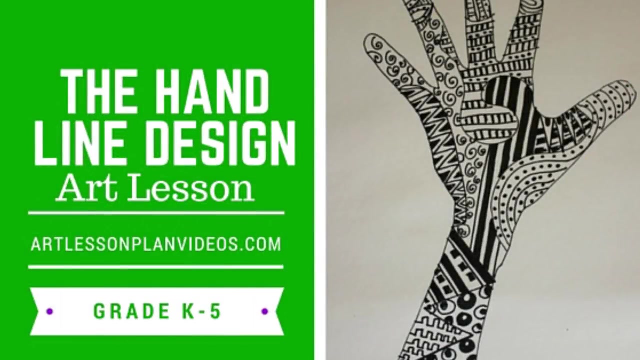 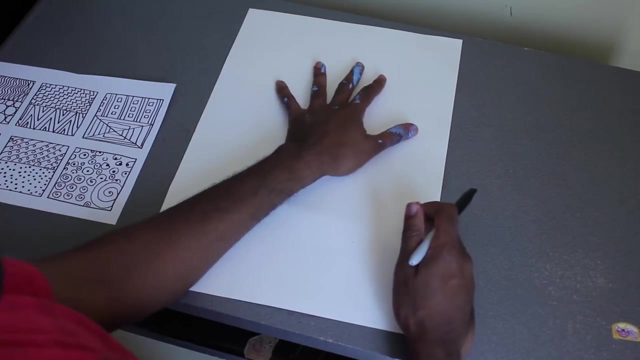 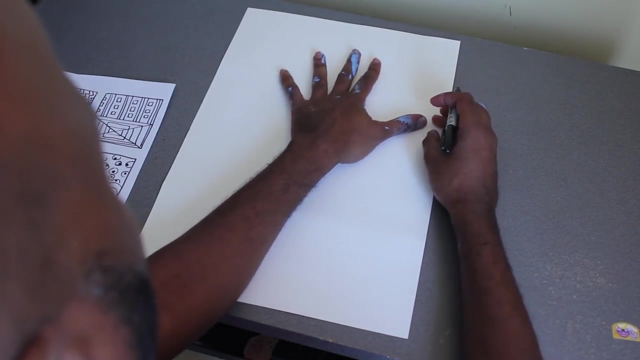 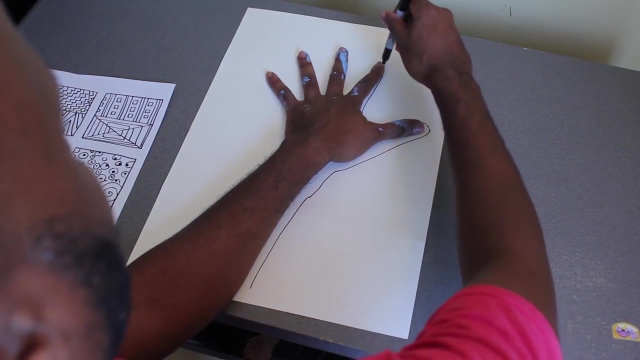 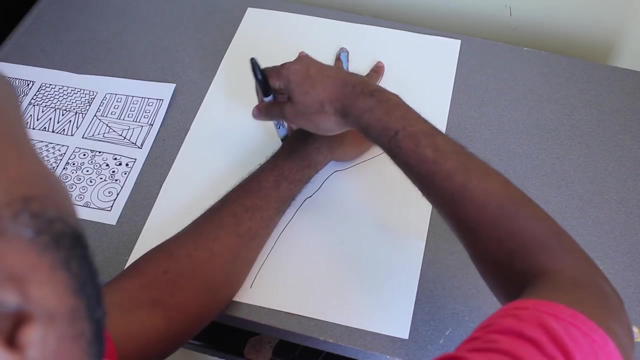 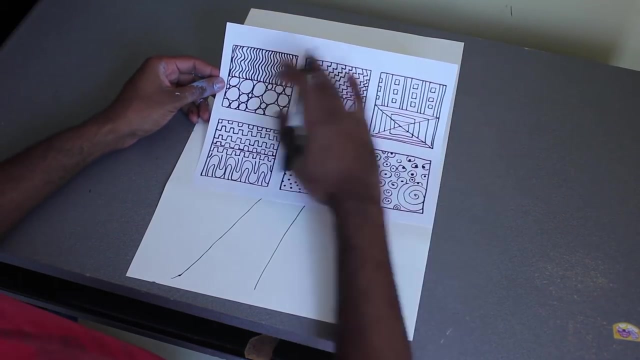 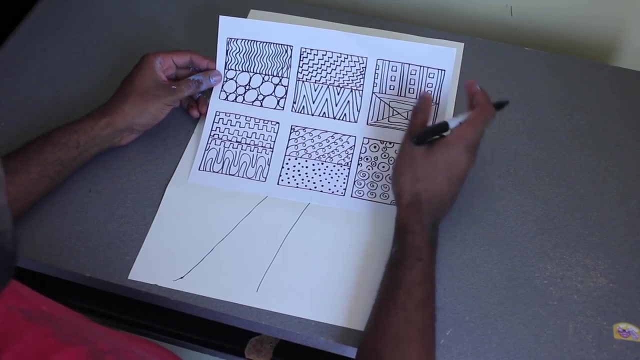 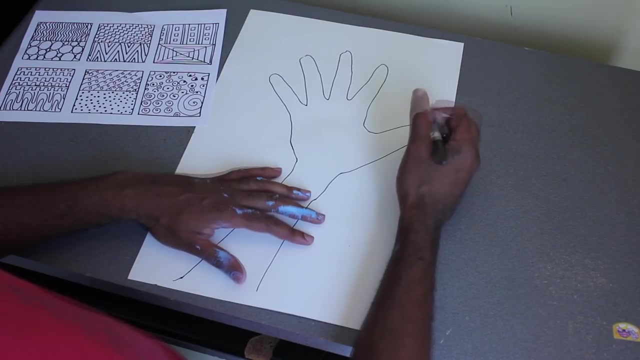 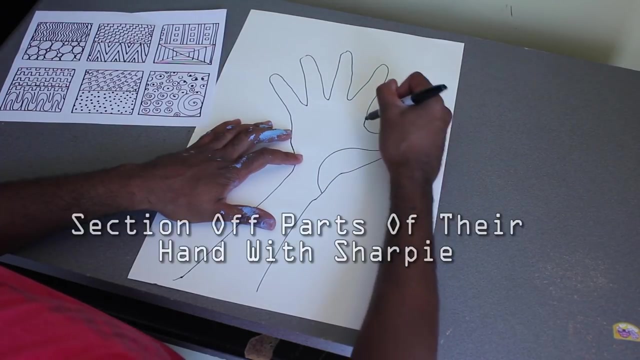 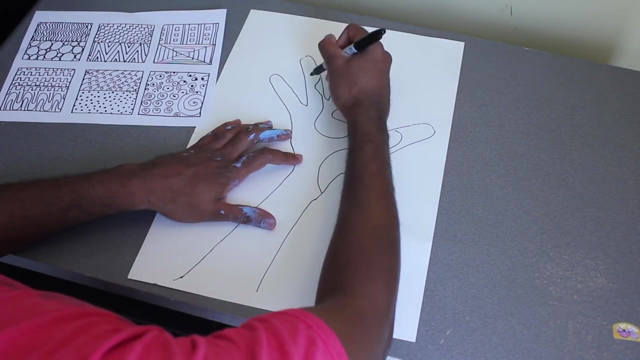 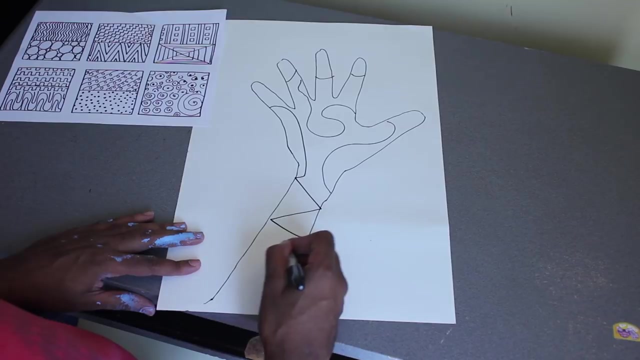 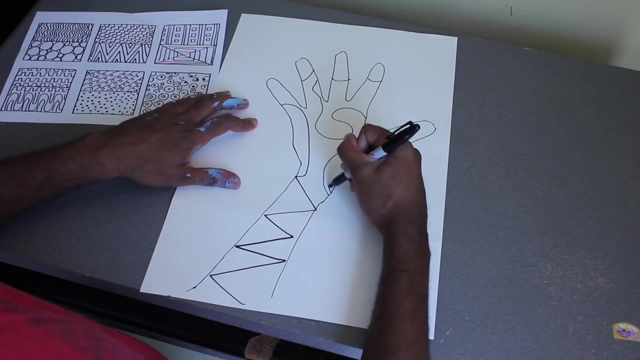 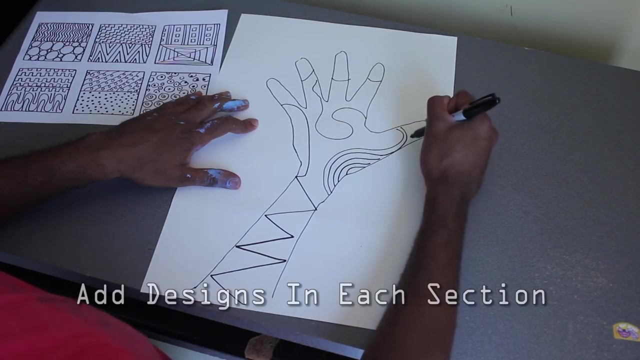 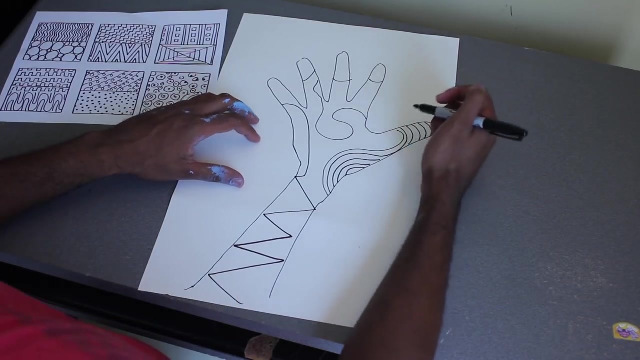 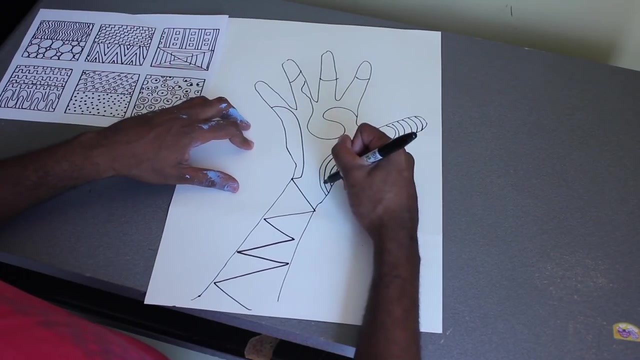 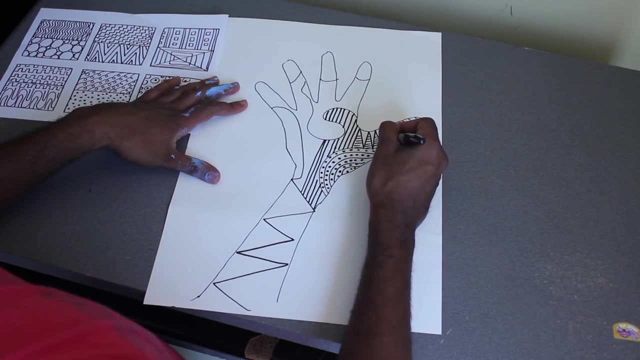 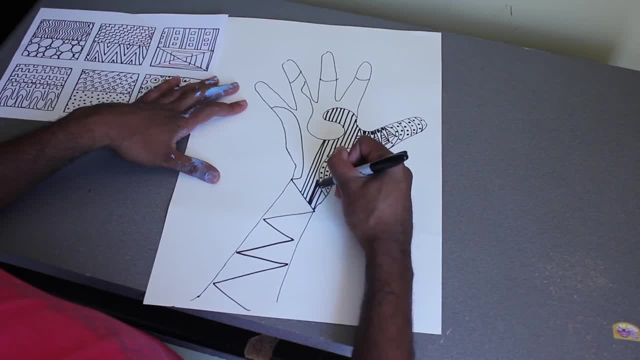 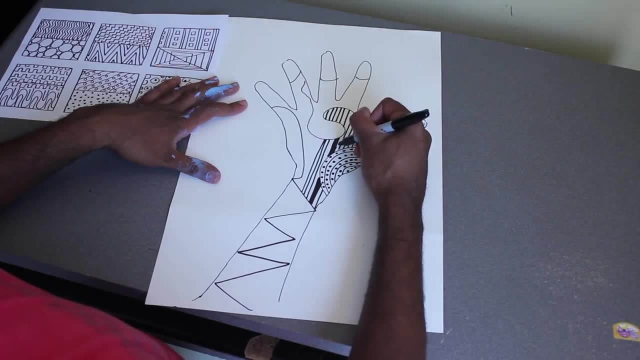 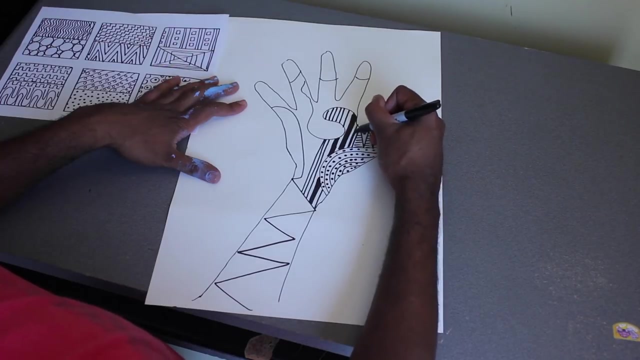 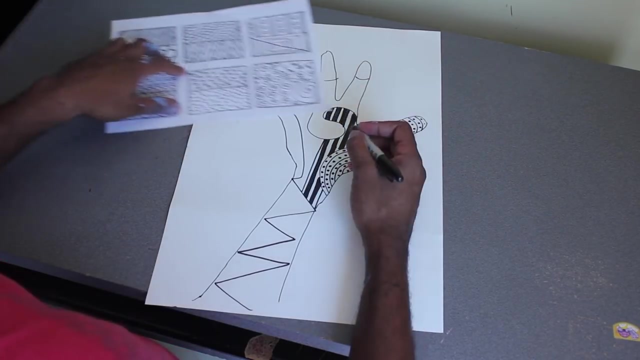 Color some of the areas dark and some of it light. For instance, these lines right here I color in dark. Skip a space. color in the next section Dark as well. I like these swirls, so I'm going to add swirls in this section right here. 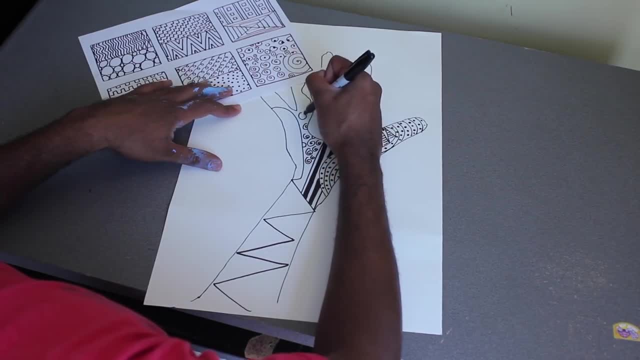 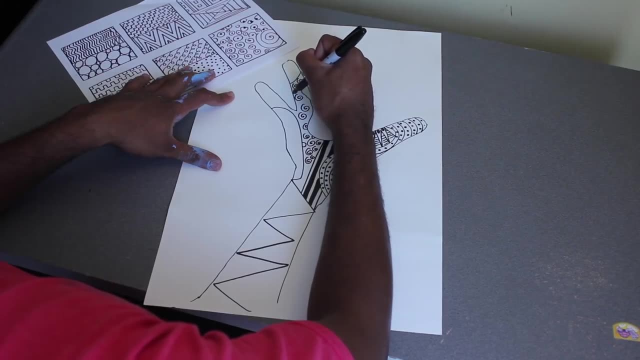 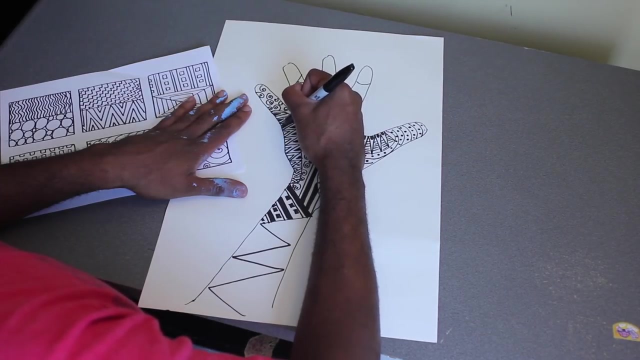 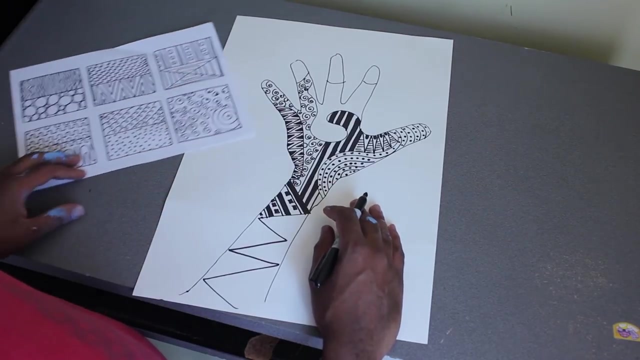